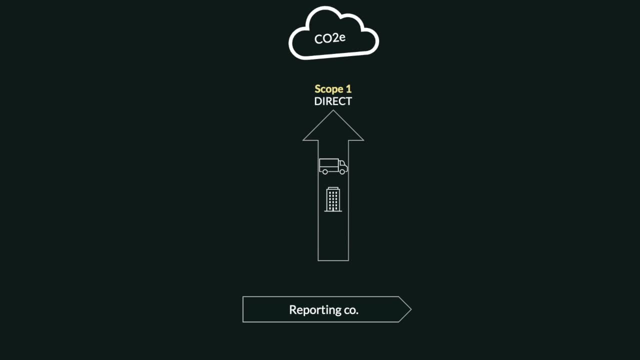 all those fuels that you burn directly. Think of this as the gas in company cars, the heating oil or fuel used to power equipment. If your company pays the fuel bill directly and owns the asset, you have Scope 1 emissions. So now let's move on to Scope 2,, which I want you to think of as buy. 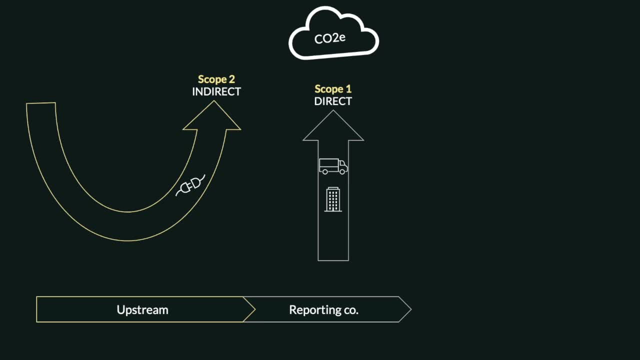 Scope 2 emissions are associated with things like purchase, electricity, steam heating and cooling, And these are considered indirect because while your company consumes this energy, it's generated off-site somewhere else, so you can't directly control it. Scope 3 emissions are indirect. 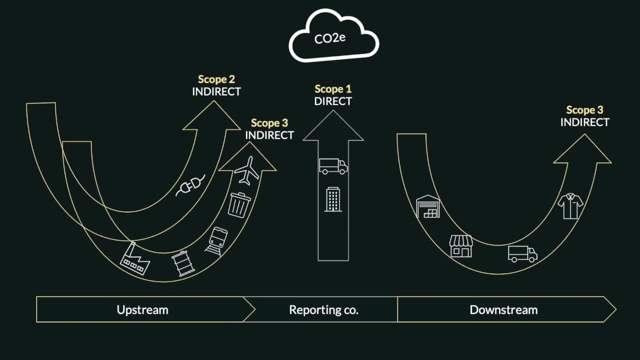 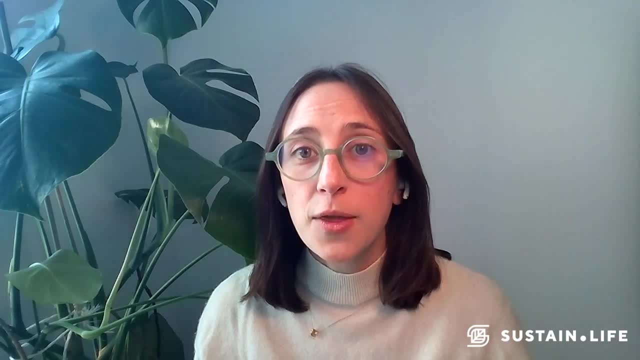 Indirect emissions are associated with everything else that supports your business operation. There are 15 categories of Scope 3 emissions. Unless you own physical assets, the majority of your emissions will likely be Scope 3.. And I have a spoiler alert: They're also the most. 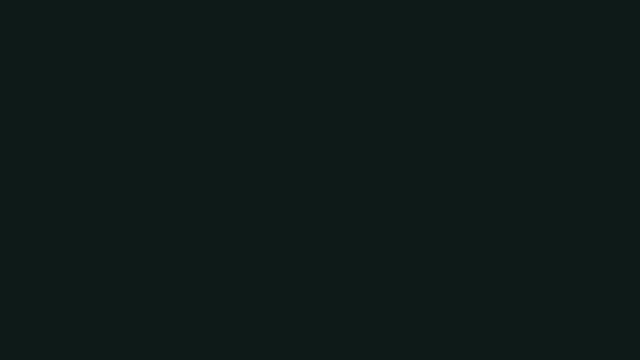 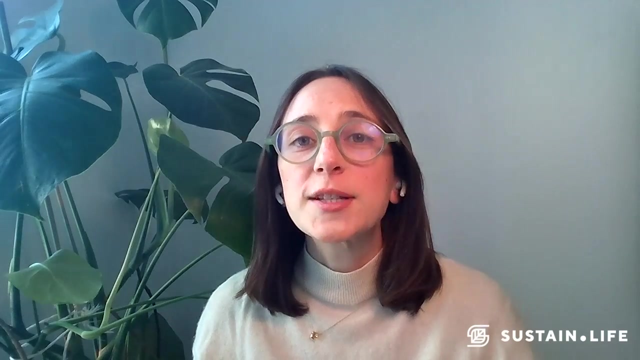 difficult to measure. So, again, a good shorthand for remembering the scopes are the three Bs: Scope 1, burn, Scope 2, buy And Scope 3, beyond. So let's bring it all together with an example. Let's think of something like this: 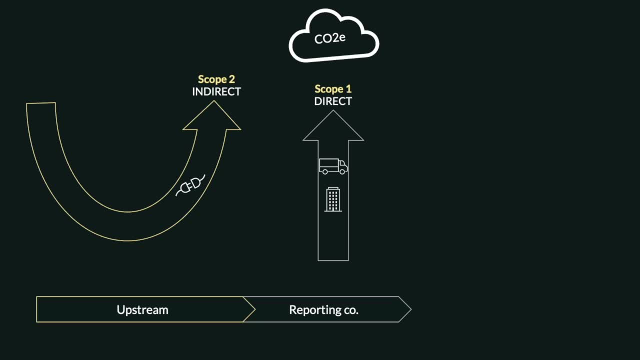 Let's think of something like a T-shirt manufacturer. They might start off by measuring the emissions associated with the energy that they use at their factories that they own. This would include, maybe, things like the diesel to power their equipment, the electricity to keep everything on the heating. 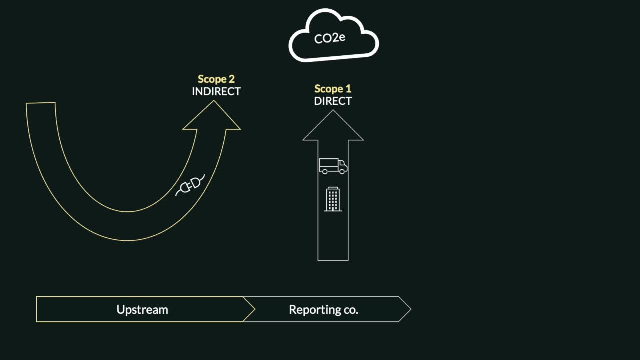 oil to keep their workers warm, And that's a great start. That's their Scope 1 and 2.. But to really understand the full impact of its business operation, it needs to look at these more nebulous Scope 3 emissions, And that includes things that are upstream as well as downstream from the point. 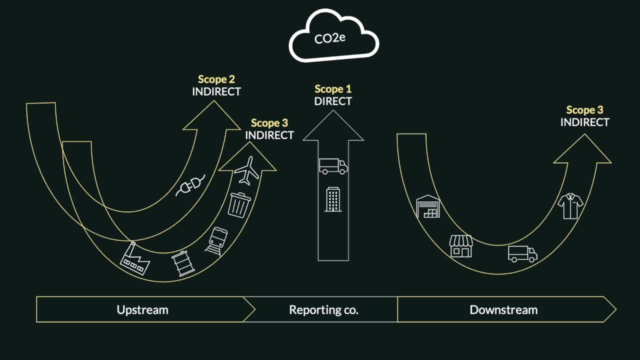 of sale of those T-shirts. So just an example of what that might include. Some upstream emissions could include the energy that it takes to process the fibers that eventually become the cotton that gets sewn into these T-shirts, as well as the transit miles it takes to deliver that raw material to the factory to be sewn into. 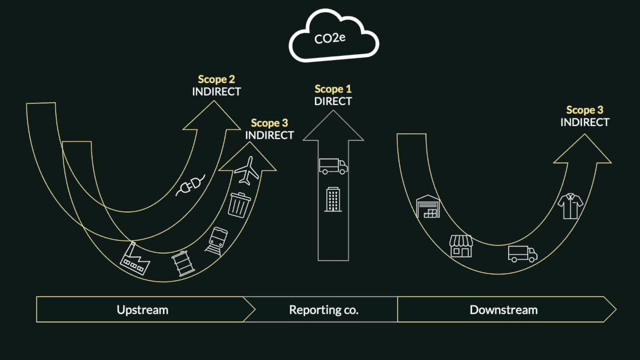 T-shirts. Those are both upstream Scope 3 emissions. A downstream Scope 3 emission could be at the end of life of those T-shirts as it decomposes in a landfill the emissions that come from that process, And that's just a sampling of what it could look like.